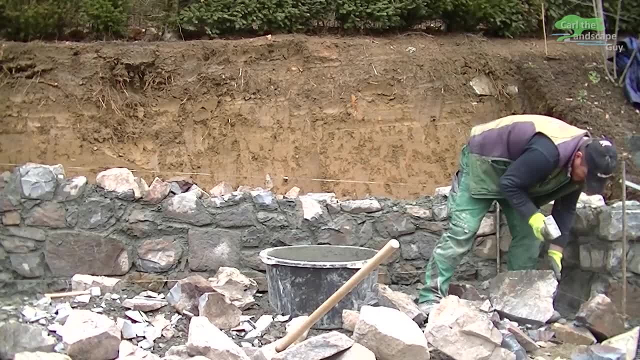 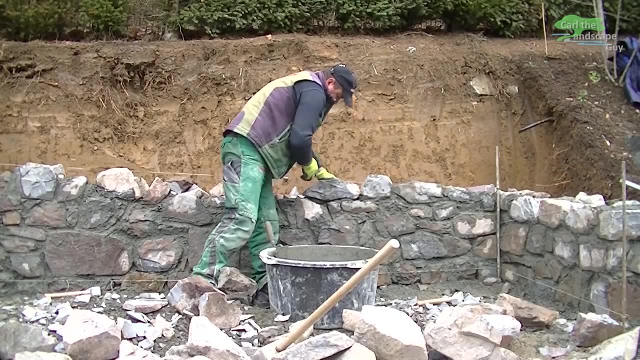 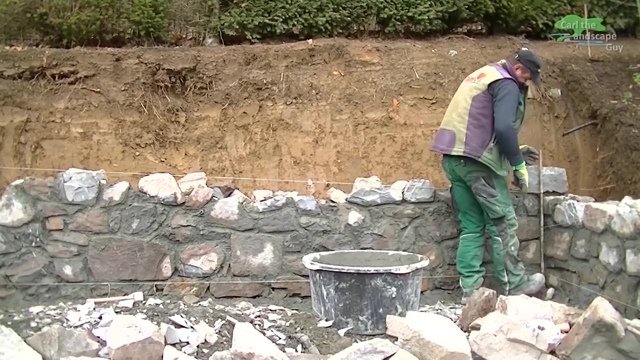 sandstone videos on my channel. But what about brittle and hard rocks? During shaping, they can break or split easily. We are with Vengelli today and he thinks you can use any kind of stone for a wall. Today's video is about a two and a half meter high and stable retaining wall made of 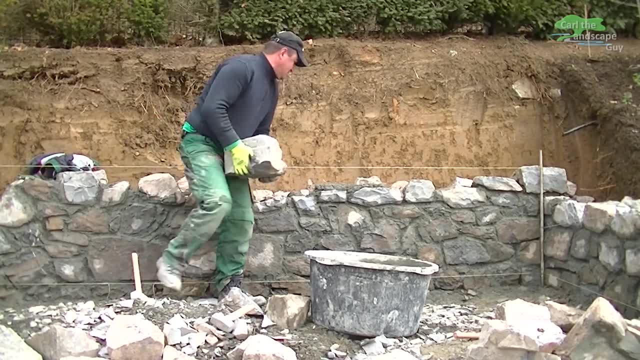 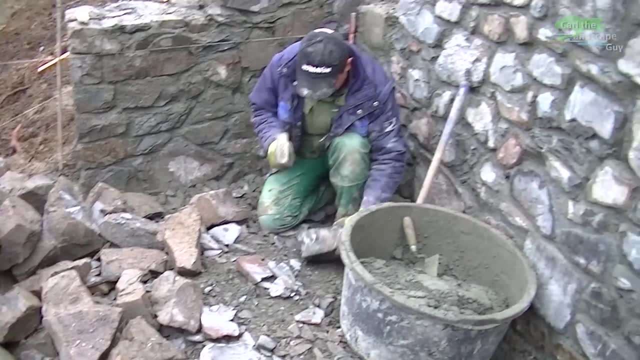 grey wacker stones, And particularly today, is about the stability of retaining walls and the progress of corner building. We're working with a really hard grey wacker stone. You can already tell that the wall will look very good, with nice light- dark contrasts. 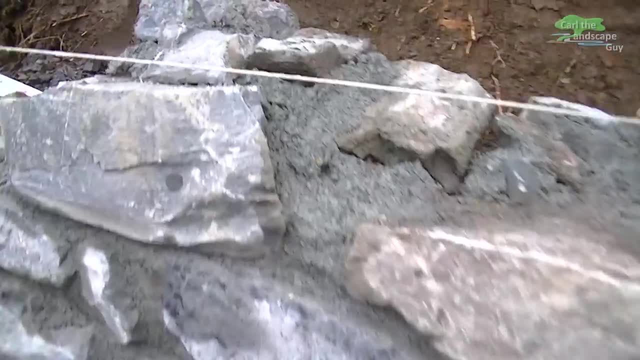 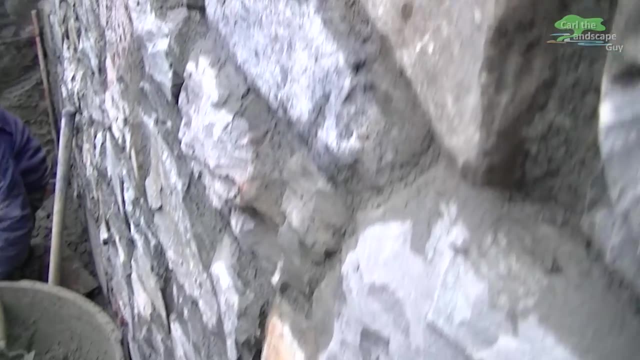 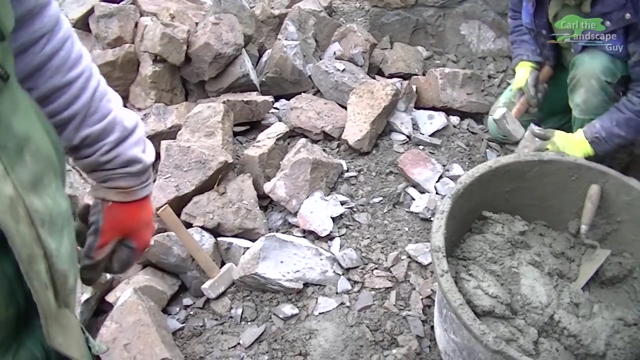 This is a retaining wall that holds very well and is stable. Without any extra concrete support behind the wall, it holds up well by using a bunch of half meter long rocks that tie in deep into the wall. This way, you can easily build walls that are three or four meters tall. 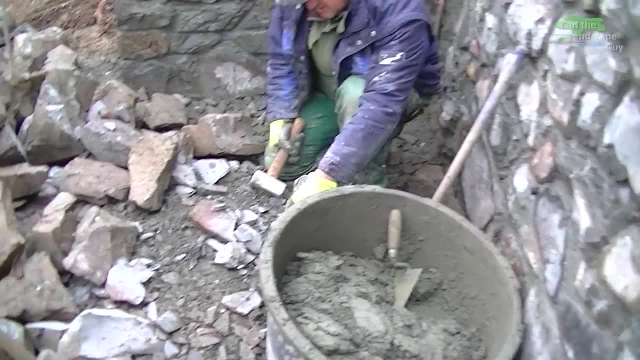 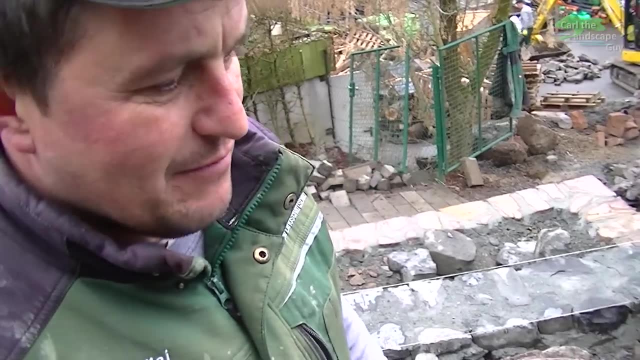 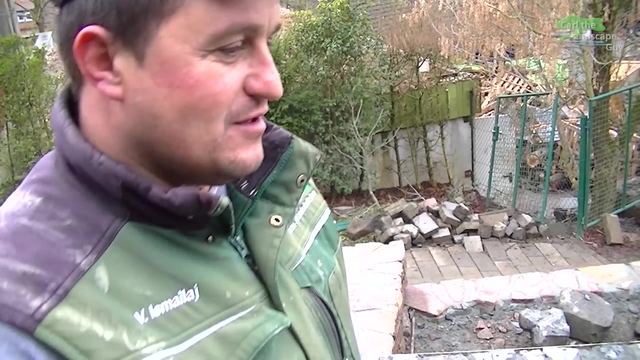 The problem with this type of stone is that it's difficult to work with, Because these are brittle stones and when you try to make a nice front or want to take away a corner, they don't break where you hit it. They can break wherever they feel like it. They already have tiny cracks that aren't visible. 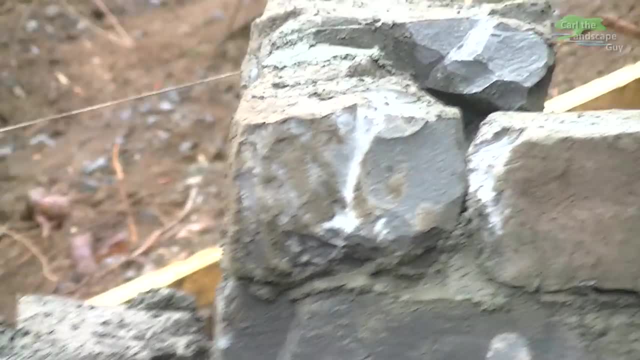 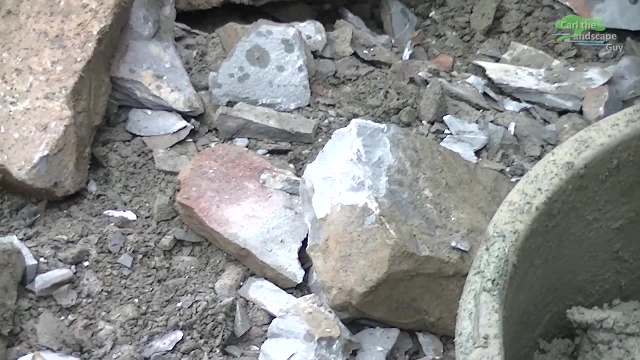 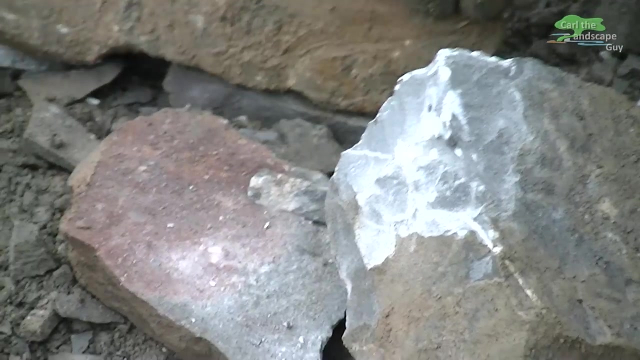 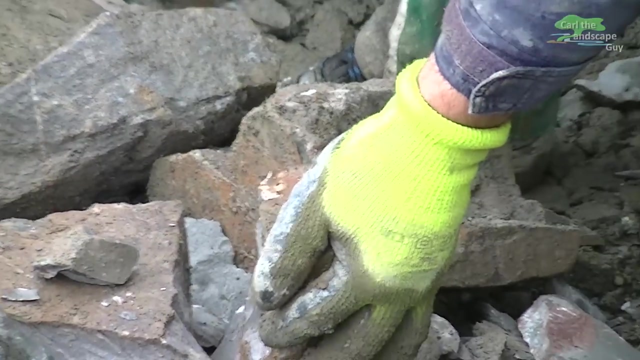 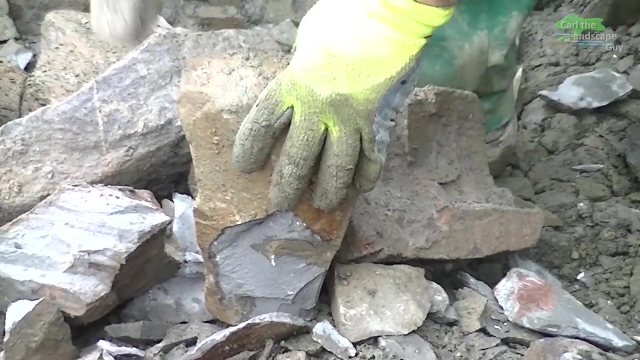 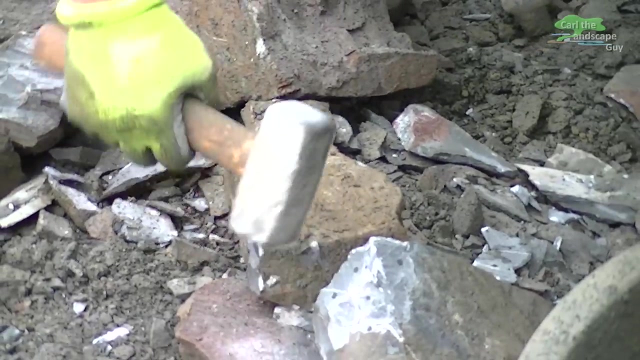 Especially, making a nice corner stone is really hard. Niko is here working on one and it could easily break apart any second. Then you can just start all over and have also lost the time you worked on it, And for this reason you want to pre-sort the stones in the quarry. 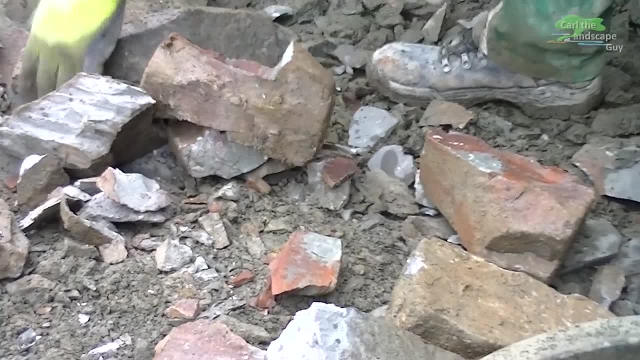 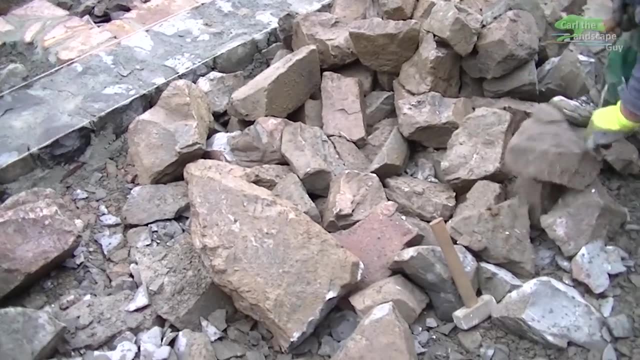 It is very worthwhile when you take a small excavator and two workers to pick the right stones. That way we can pick and prepare about 50 vertical square meters of wall per day. Then we load them onto our truck and bring them to the construction where we build the wall. 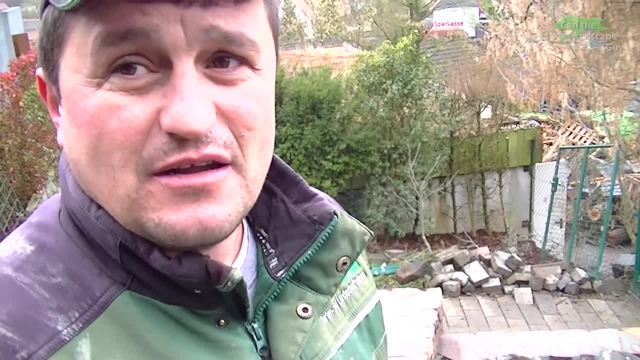 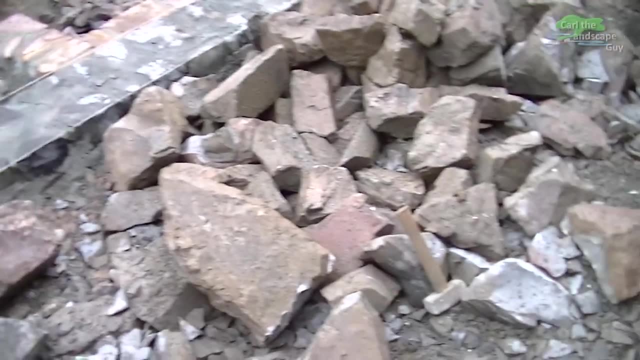 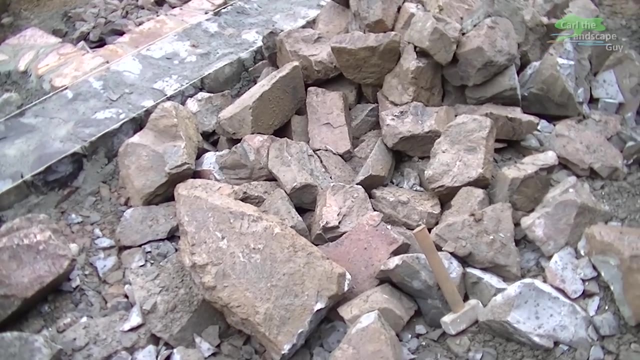 The good thing is we only have stones at the construction site that are really usable, and not that many waste stones. Otherwise, we're talking about 30% rocks and gravel that are not usable. Here we can use it as backfill material, But that doesn't work on every job. 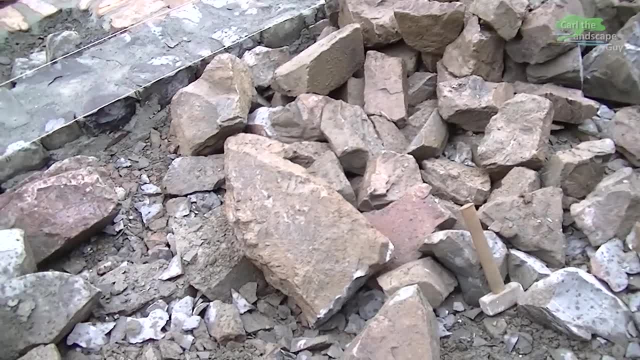 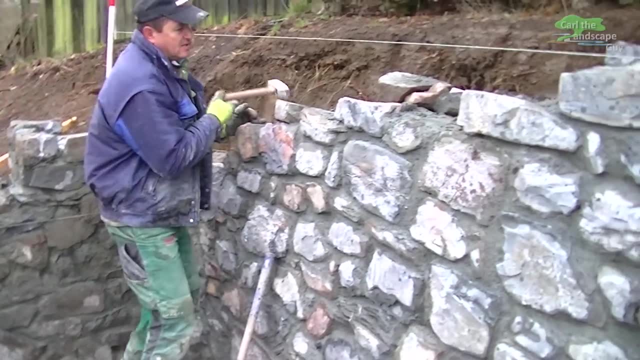 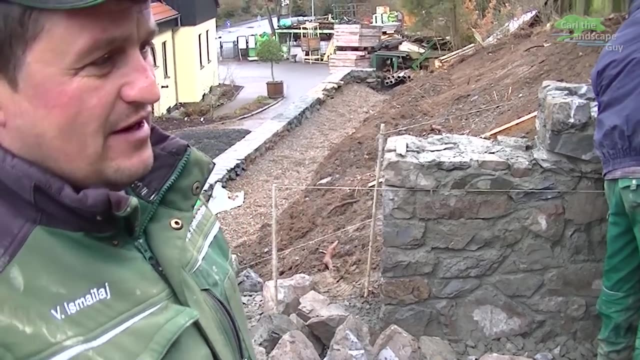 Because here we have our retaining wall that needs to be backfilled. If we have a two-face cladding wall, for example, we don't have any space to put the waste material. Then picking it back up and getting rid of it takes time and money. 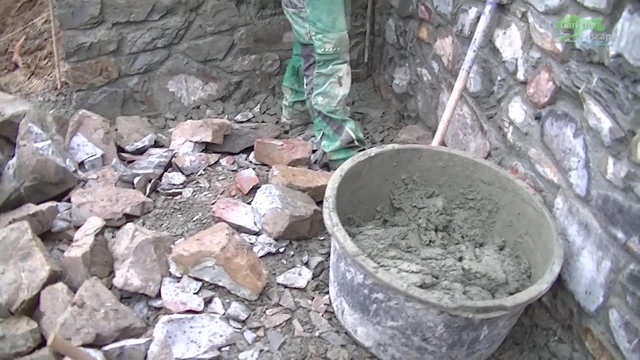 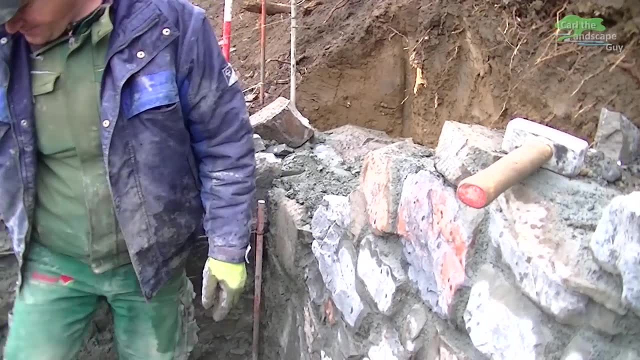 Therefore it is better if we pick the stones ourselves. That way it's also easier to plan, because we could go and say, okay, we need 100 cornerstones. Then we can take our excavator with the grabber attachment and pack the stones we need. 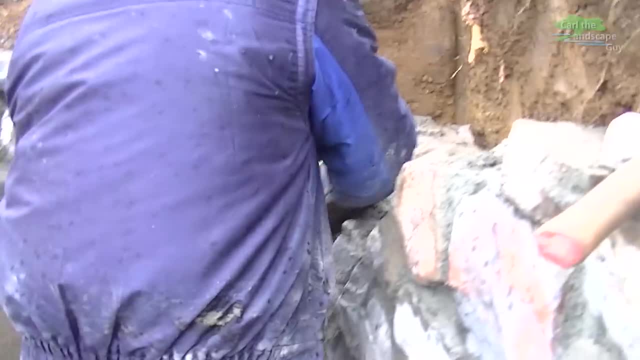 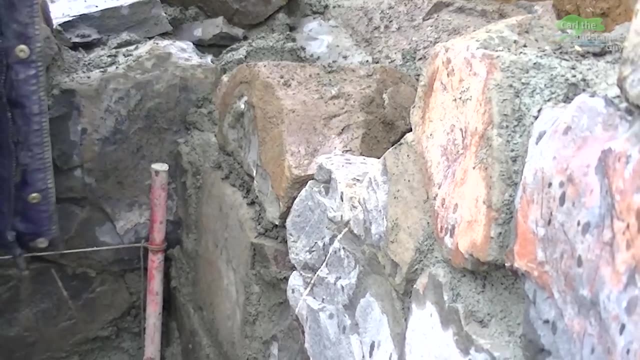 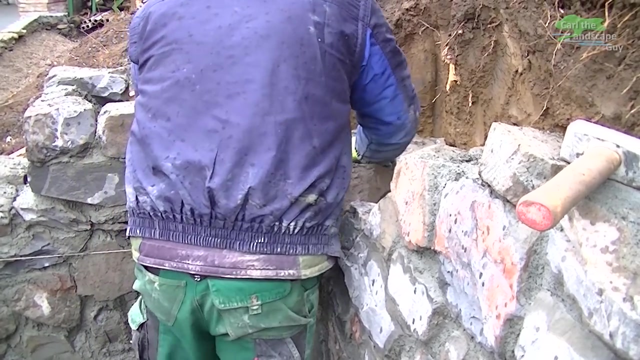 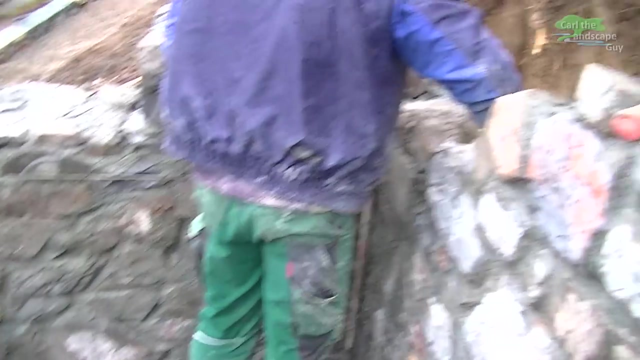 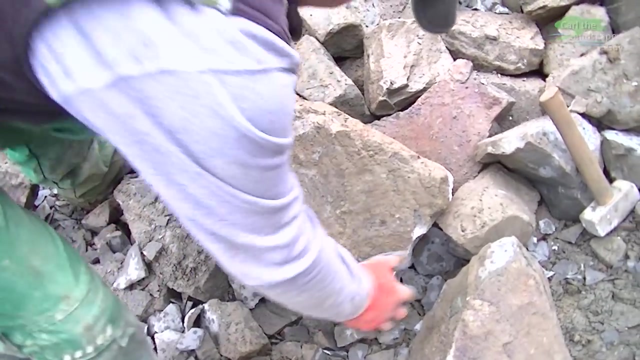 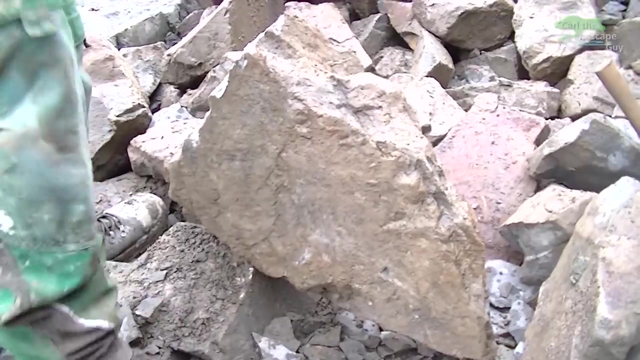 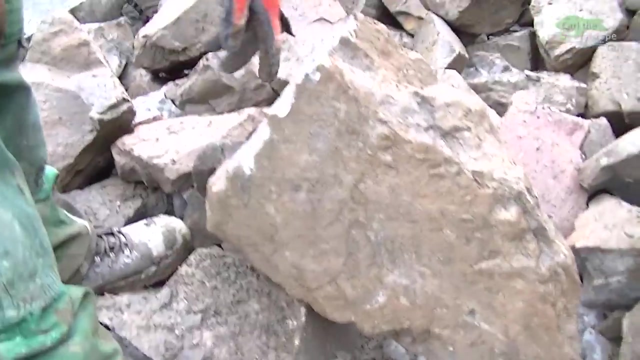 With the time we lose there in the quarry we can do at least two more square meters of wall per day. We can add one to each of them. Here we have a nice big stone. It has a nice face here. But of course we can not put it in like this. 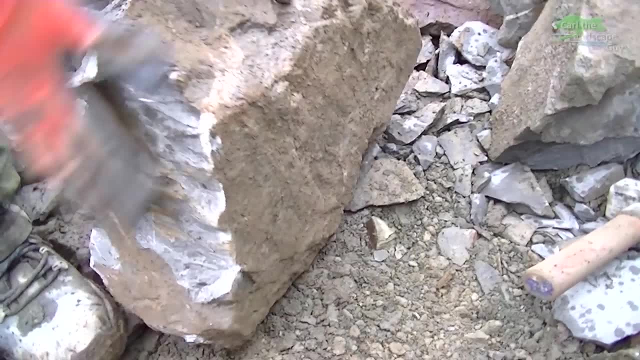 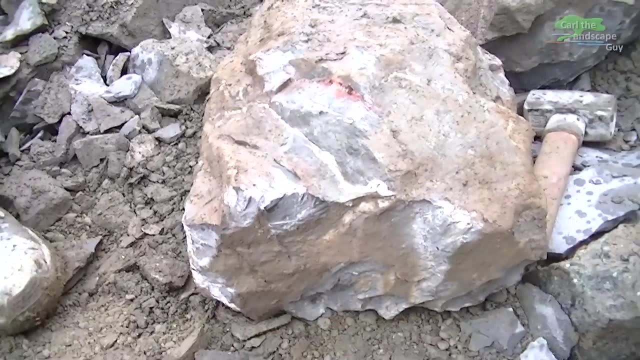 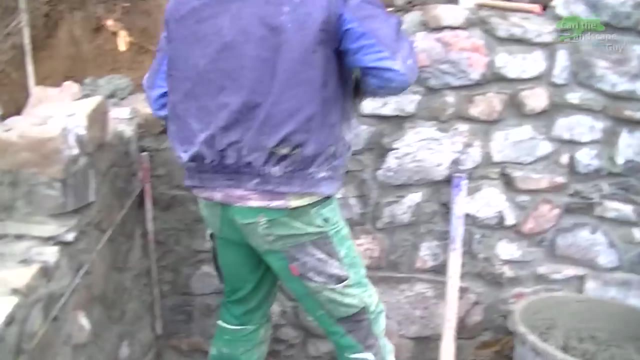 You could put it like that, but definitely not in the retaining wall. We prepared a face on that side and we can set it in the wall. now We will put it in so that it ties deep into the wall. That, combined with the motor, will make the wall very strong and retains 150 tons on the 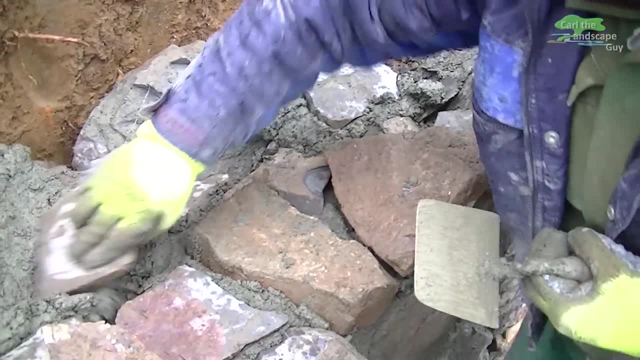 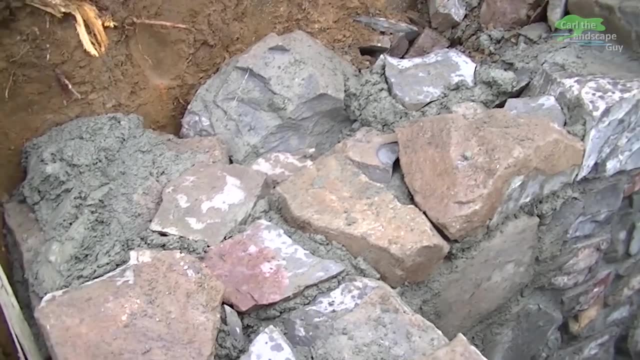 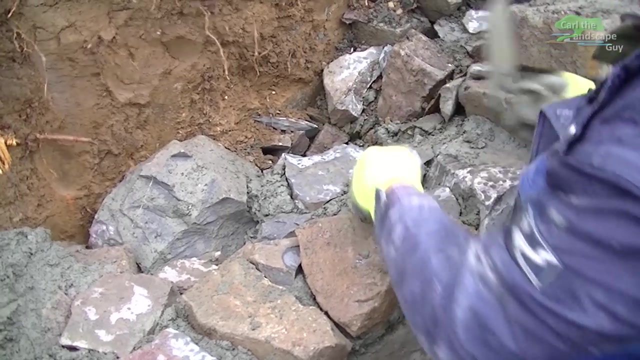 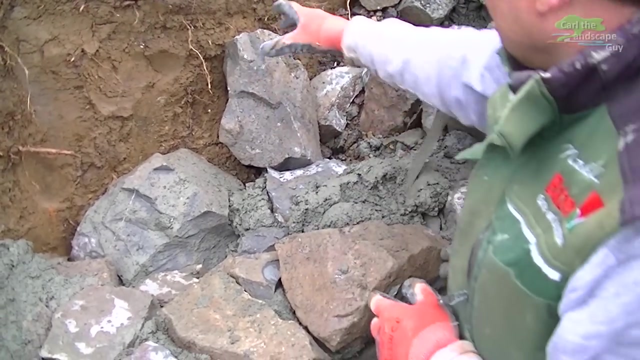 other side, no problem. It is also important how we pack the stones in the back. The stones should also be packed properly here and not just thrown in. We close the gaps- at least 80%- with mortar. The stones must definitely be laying like that. 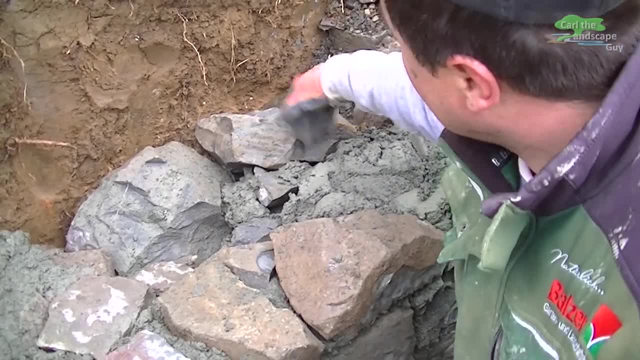 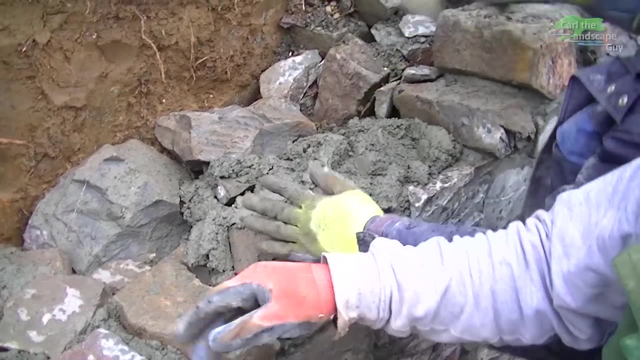 We do not need any mortar in this drainage area. Up to here is the mortar And behind it is the drainage area without mortar. 40 cm of mortared wall and the rest doesn't need mortar behind it so that water can run down later. 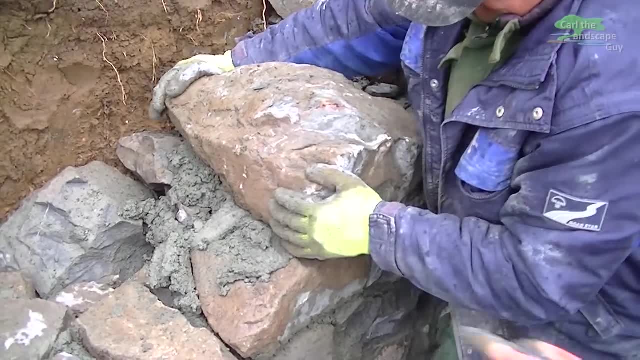 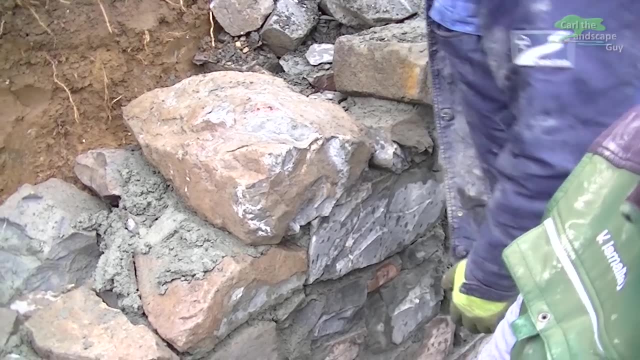 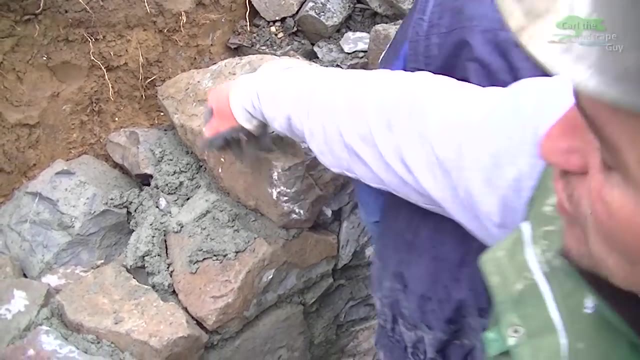 For each vertical square meter of wall, you need at least 3 big rocks with this length that tie in deeper. The deeper the better. If the wall is 3-4 meters high, we have to start at the bottom with the biggest stones. Of course, this is only possible when the wall is 3-4 meters high. 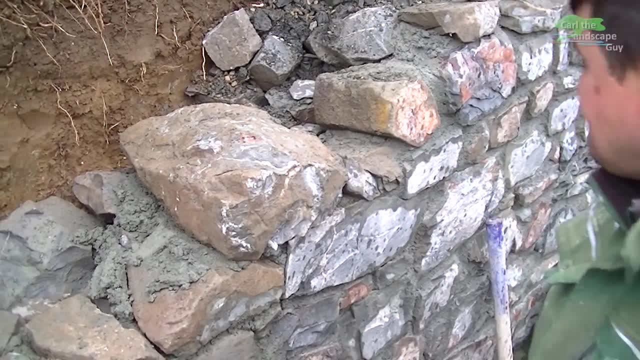 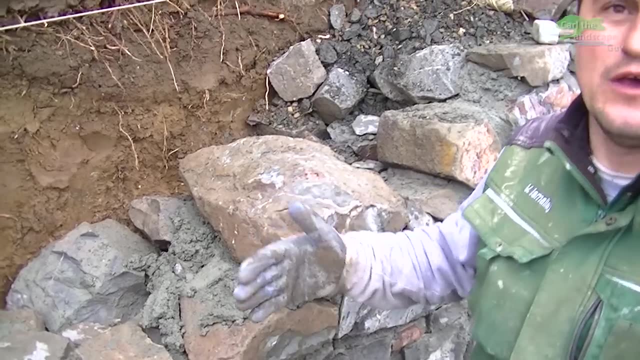 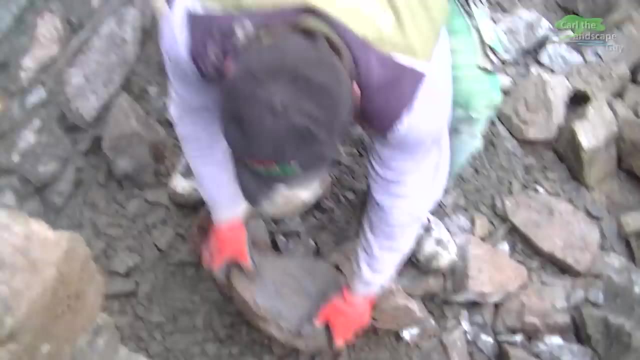 If the wall is 3-4 meters high, we have to start at the bottom with the biggest stones. You can also start with a wall with an appropriate wall thickness or, like here, a retaining wall. If the wall comes to such a height, then you have to use big stones. 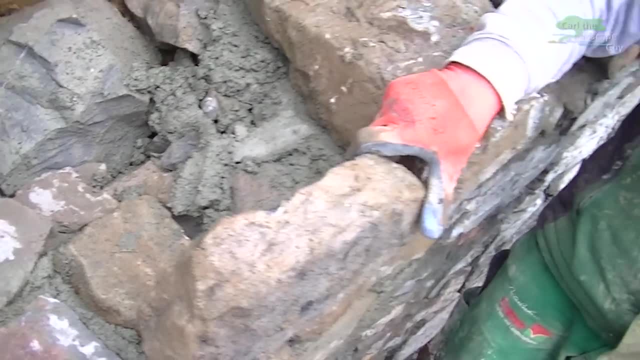 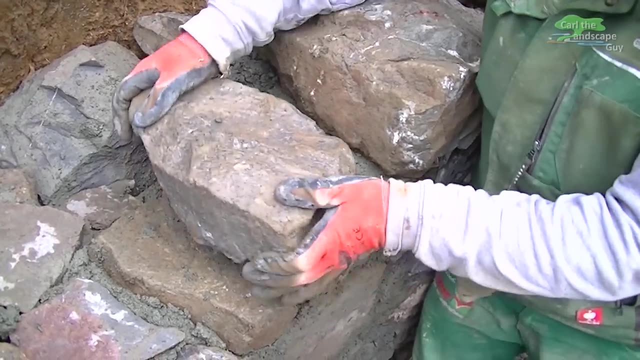 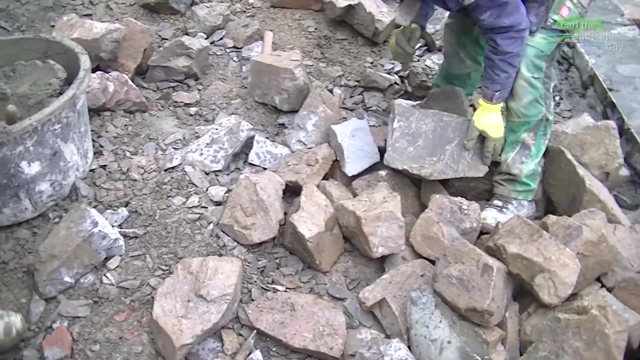 Because such a stone cannot be walled like this. that's not possible, In no case, even if it's twice as wide. I wouldn't put it in that way. I would put it in like this: So mortar with it Then in this way. 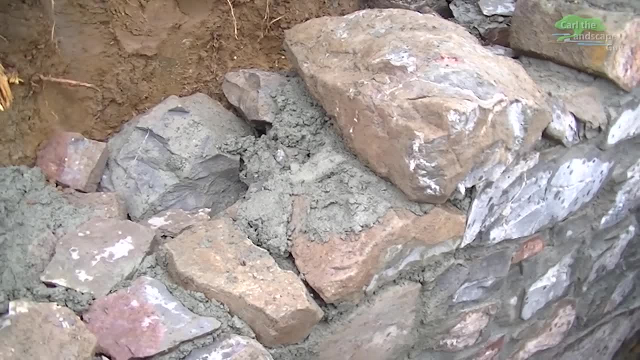 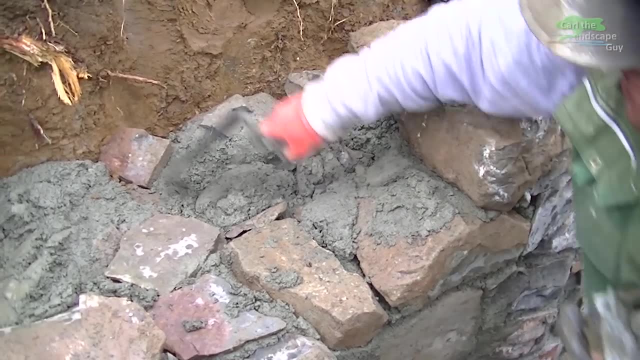 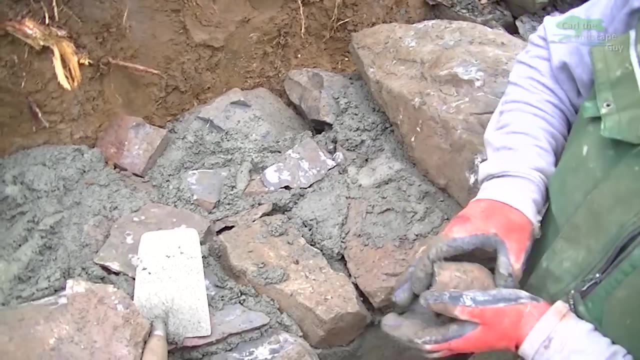 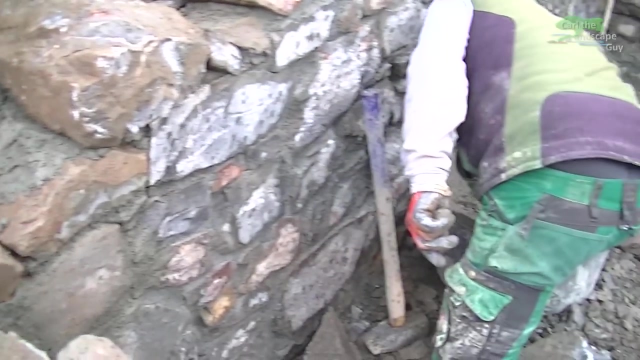 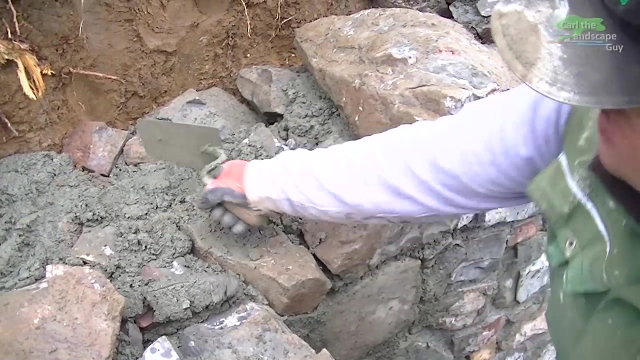 Then we take the waste, rocks and gravel Here. it is good that we have it because you can fill the gaps nicely with it. We put some mortar and then you can let the stone swim like that. Now we set this inside cornerstone. Now you might think: why this way? 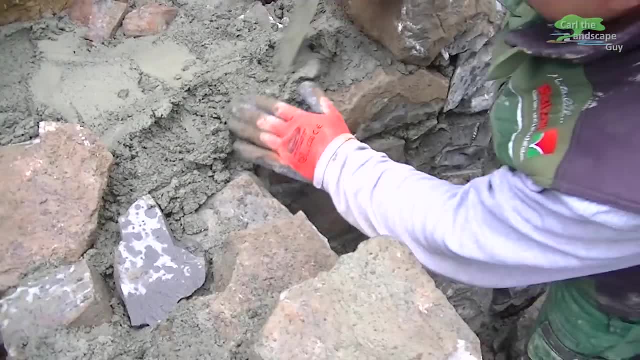 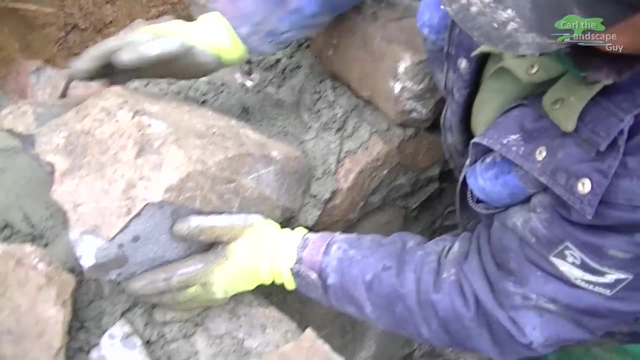 Well, because half of it will disappear later and the rest of it will be gone. But that's not the point. The point is to make sure that the stone is in the right position, And that's it. Now we can start with the cornerstone. 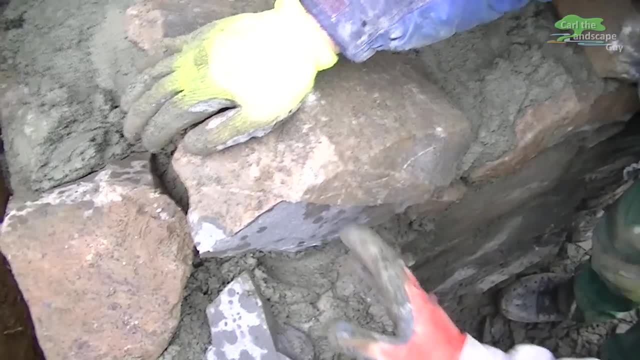 Now you might think, why this way? Well, because half of it will disappear later and the rest of it will be gone. But that's not the point. That has to go like that, Because otherwise we can not make a proper vertical grout in the corner. 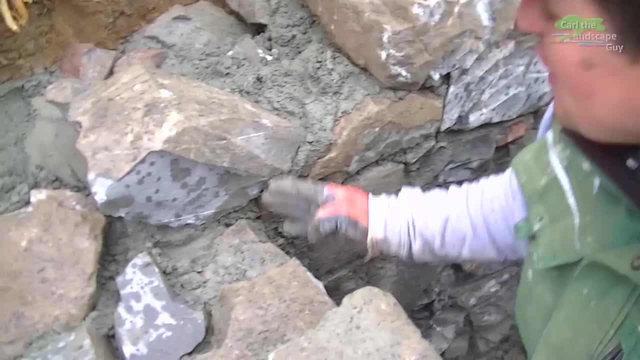 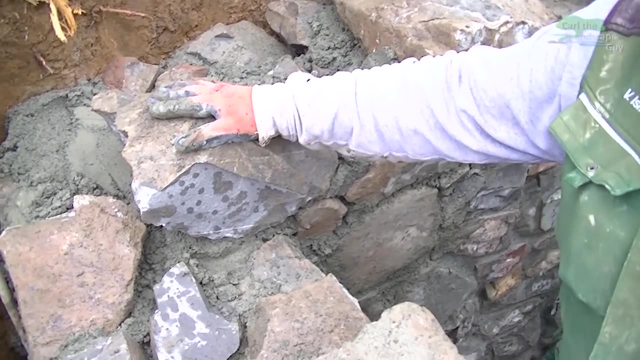 We don't want the two wall parts to move apart from each other. Not every layer has to be that way, but we do like every third one. Also, keep in mind that it should not be too cold or too wet when building your wall. 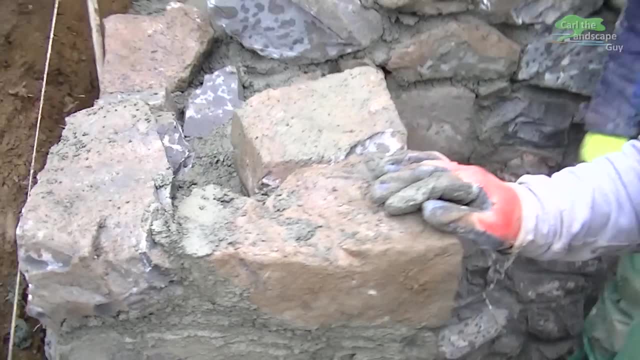 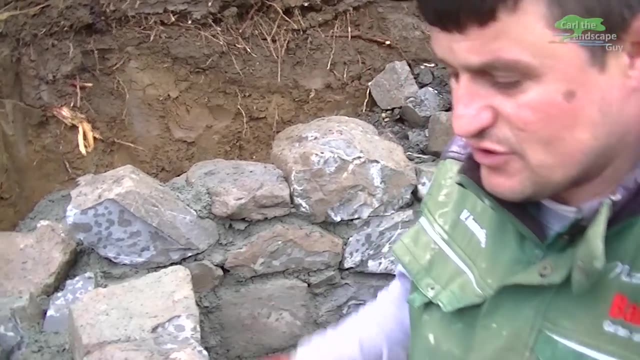 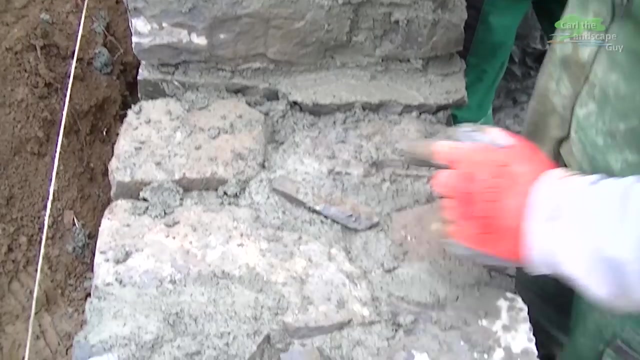 We stop building when it gets colder than minus 3 degrees celsius. Then we cover the wall up with fabric overnight. But when it rains, the problem is that the stones are wet and the greywacker stones don't draw any water. The mortar doesn't thicken up by itself and since the rocks don't draw any water, the